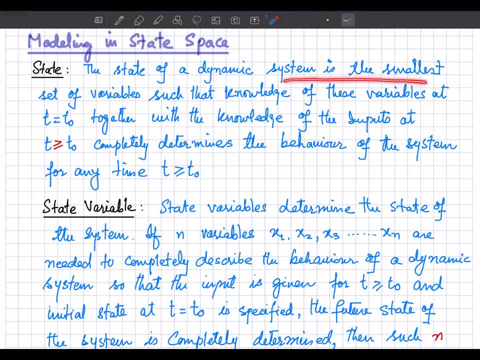 A state of a dynamic system is the smallest set of variables, such that the knowledge of that variable at time t is equal to 0, together with the knowledge of the inputs at that time, that is, at time t is equal to 0 or at any other time, t greater than t0 completely determines. 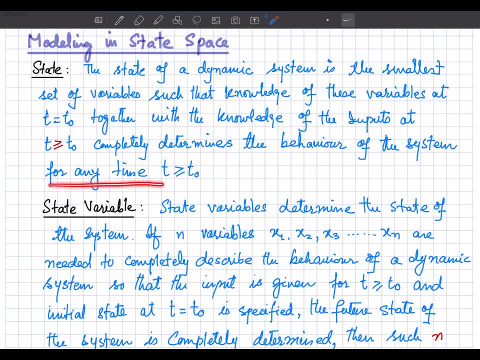 the behaviour of the system for any time, t greater than or equal to t0.. So a set of variables with the help of which we can determine the future state of the system for any time is called the state variable, And all of these state variables define the state of the system. 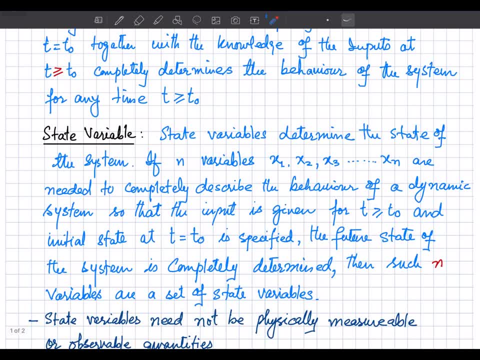 So state variable determines the state of the system. and for any system, let's suppose that there are n number of variables which are required to describe the behaviour of of that dynamic system. so if you know the information of the inputs at that time or at time t greater than or equal to 0, and you know the initial states of 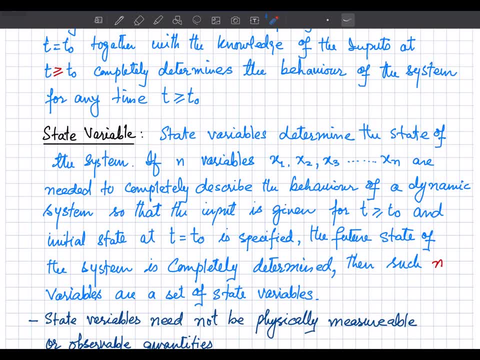 those selected variables x1, x2 or x3 up to xn, if you know their initial states at that time, that is, at time t is equal to 0. that is specified. the future state of the system is completely determined. such n variables are called the set of. 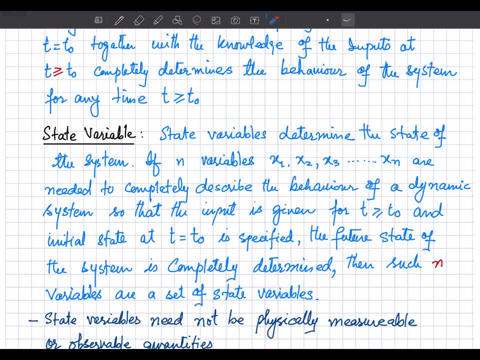 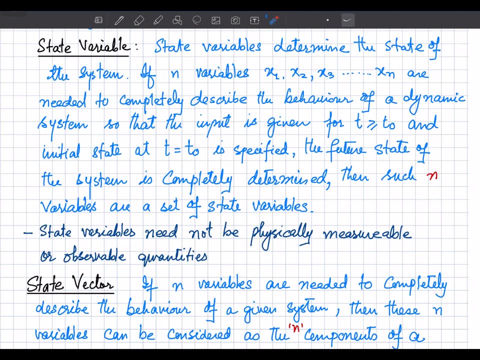 state variables. these are the state variables- define the behavior of your system if the input is known at a particular time. okay, for example, the state variable for the inductor is the current. if you know the current at given time, let's suppose t 1- and if you know what is the input at that time, 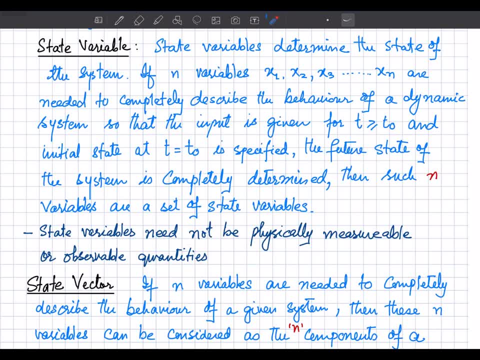 instead of time. you can determine the current, in the future, at the time t greater than or equal to zero. similarly, in the capacitor the state variable is the voltage. so state variable may be a physically measurable parameter or may not be a physical measurable or observable quantity, but usually we select the state variables which are measurable so that we can easily define the 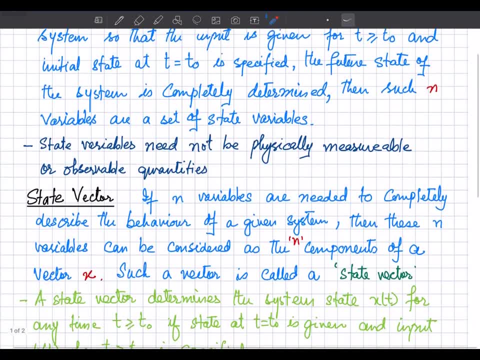 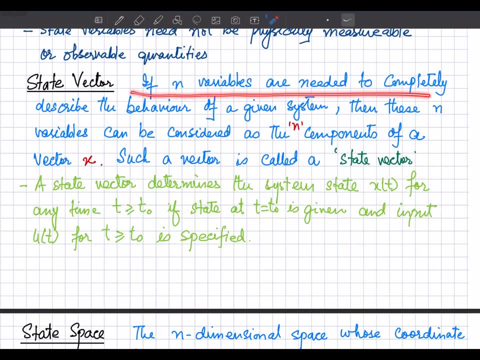 control system. okay, now let's talk about the state vector. if n variables are needed to completely describe the behavior of the system, then these n variables can be considered as the n components of a vector x. so as these are the state variable, so this vector is said to be. 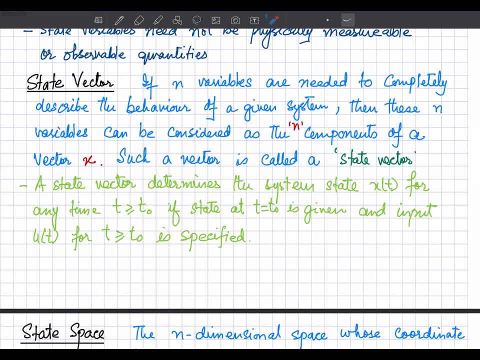 the state vector. so a state vector determines the system state. let's suppose that is x of t for any time t greater than or equal to t 0. if state at time t is equal to t 0 is given and the input g of t for time t is equal to, greater than or equal to t 0 is specified. 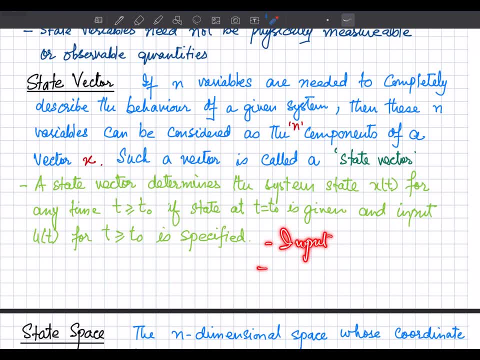 so if the input is known, if you know the input and if you know the initial state at a certain time, t naught you can define, you can determine the future state of the system. so a vector state vector is basically a vector which consists of the n state variables. 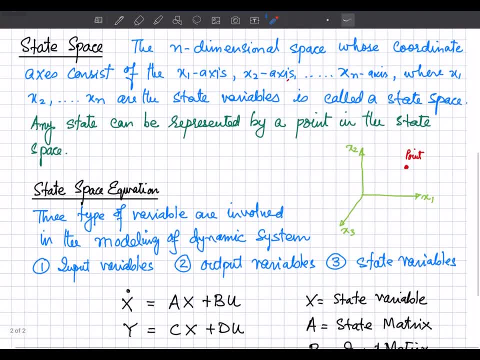 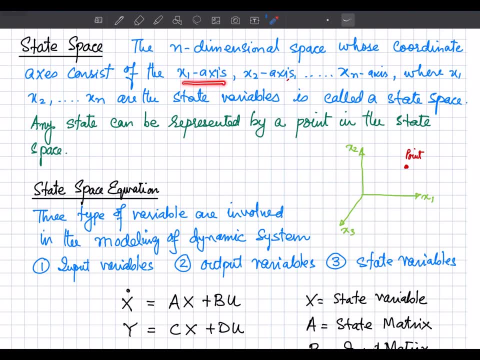 okay, now let's define the state space, the n dimensional space, whose coordinate axis consists of the x 1 axis, where x 1 is the state variable, x 2 axis, and so on up to x and x, is where x 1, x 2 and x n are the state variables. 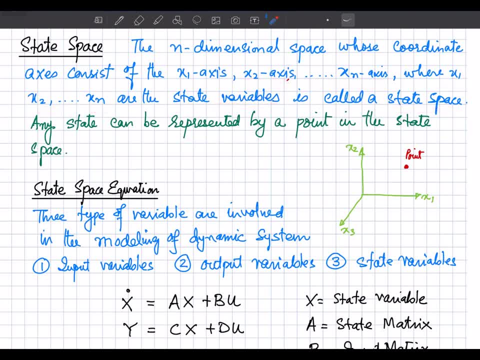 the state space, so a state can be represented by a point in the state space. just for the sake of example, consider the set of the x's. let's suppose this is the x1 x's right, this one is the x2 x's and this one is the x3 x's. so a point in this will define the state of your system and definitely 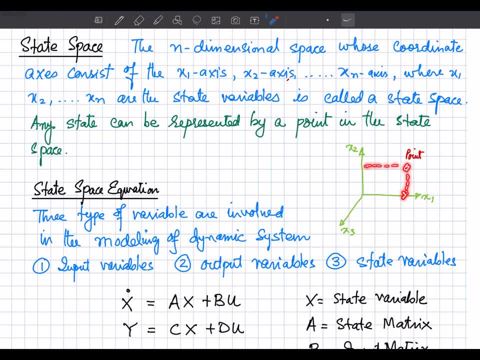 and it will be a function of x1, it will be a function of x2, it will be a function of x3. so in n-dimensional space, a point, define the state of the system and in that space, your state variables are basically the coordinate x's right. okay, now the system is defined. 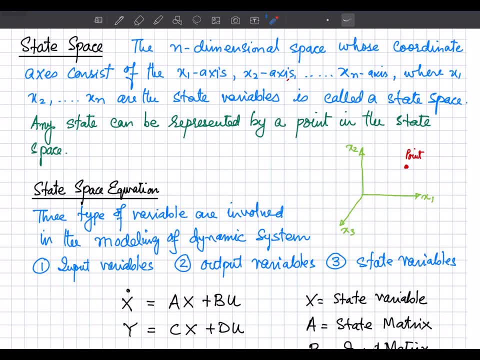 usually with the help of the differential equation or the transfer function, so the directly related definite constant. and so, for the sake ofаю, then, we have seen that the state of the system is defined as x, and so that's what we are going to talk about today. 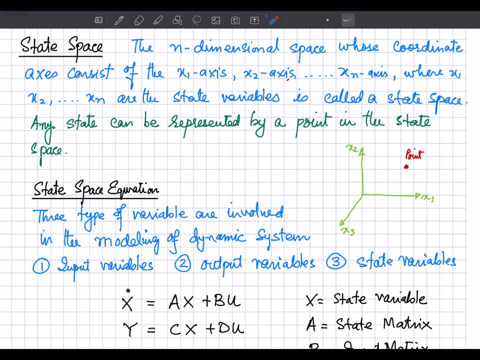 we can translate the differential equation and the transfer function in terms of state space equation. So what is the state space equation? Basically, it relates your inputs and outputs using the state variables, right? So three types of variables are involved in the modeling of the 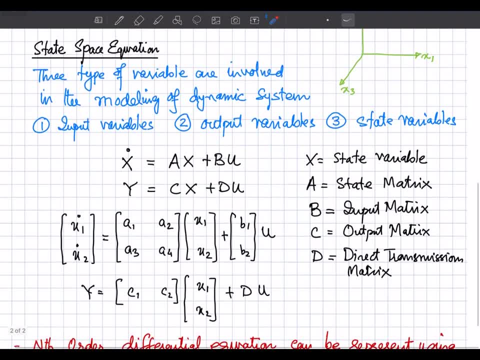 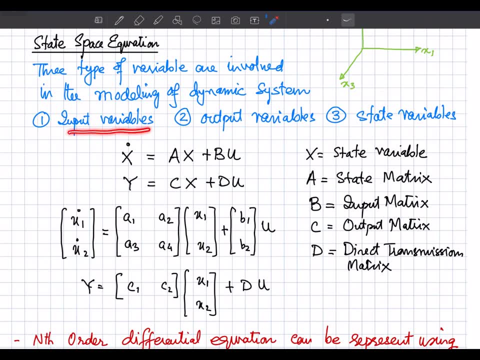 dynamic system. The first one is the set of input variables, the inputs of your system. The second one is the set of output variables and set of state variables. So, in generic, the state space representation of a system is given by this set of equation. where this is, 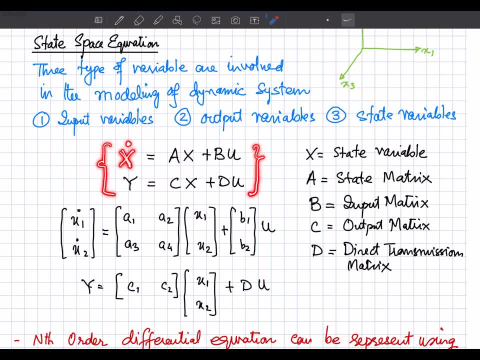 representing the derivative of the state variable right And in this case the state space equation. A is the state matrix, this one. this may be a function of time, but usually it is constant for an LTI system. B is the input matrix, U is the input of your system. X is the 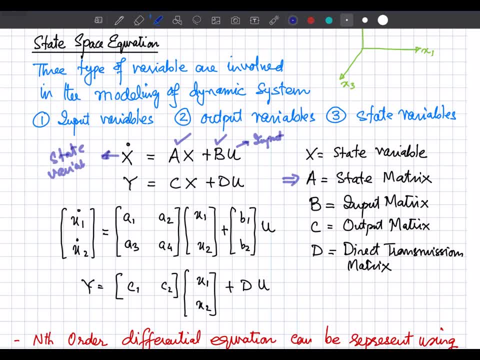 state variable Y is the output of your system, C is the output matrix right, d is the direct transmission matrix and the u is the input. okay, so what this x is representing? this is basically representing a state variable vector in which there are n state variable components. okay, so this set of equation can be written like that. let's suppose that this: 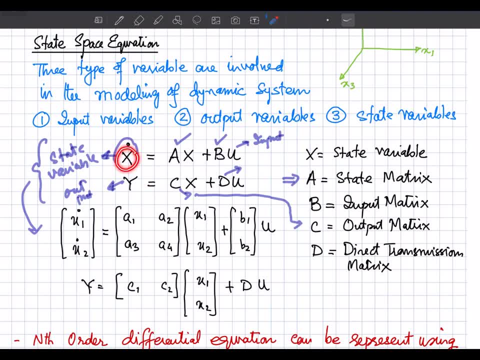 state variable x is consisting of two components, x1 and x2, and this is the vector and these are the components of this one, x1 and x2. so this dot is representing the derivative. so x1 dot, x2 dot, let's suppose, is equal to some matrix: a1 into a1, a2, a3, a4, and this is multiplied by the state. 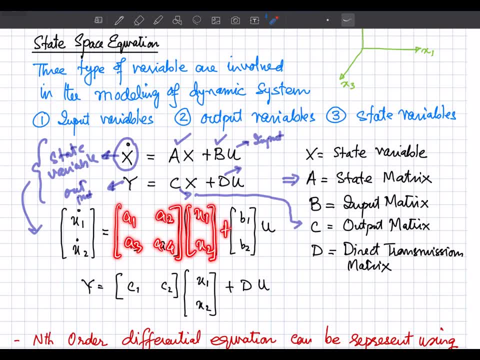 variable vector, again plus b1 and b2, and there are two components in this and this is the input. so similarly, the output equation can be written like that: y is the output, that will be equal to c1 and c2 and this is the matrix c multiplied with your state variable vector. so x1 and x2 plus d into u. so 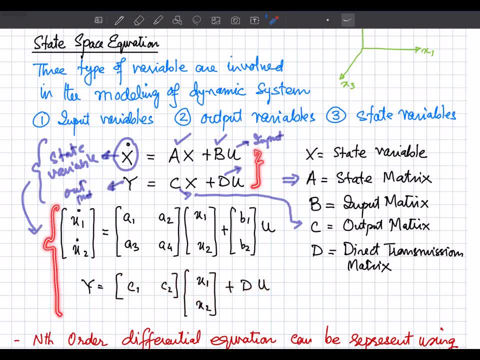 this set of equation can be written like that: there may be the three state variable, there may be four state variables, so other of this metric matrix will be equal to the number of state variables. and 2 cross 2 matrix for two state variables. 3 cross 3 matrix for three state. 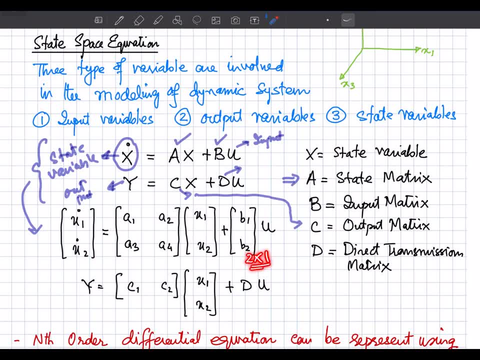 variables. similarly, the order of this one to cross, one for the two state variables, three cross 1, 4, 3 state variables, and so on, and if their end multiple inputs, you can have the number of columns as well, more than one columns, okay, so what basically state space is. state space basically represents your nth order. 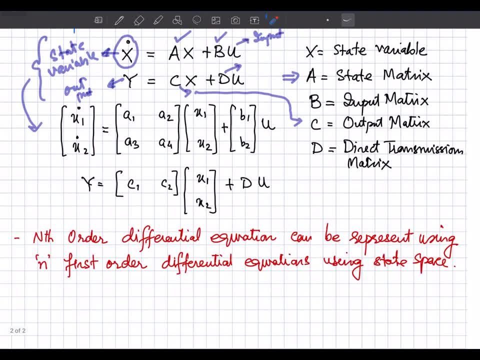 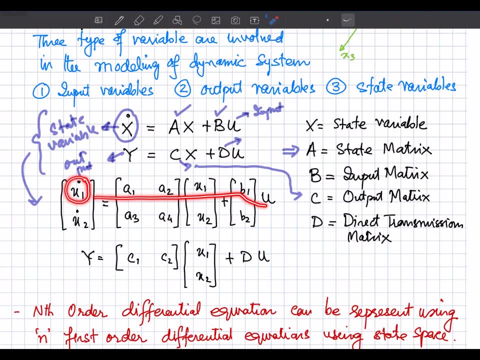 differential equation with the help of n, first order differential equation. so here you can see, there is only, you know, first order derivative in if, if i define an equation with the help of this row over here. so this is the first order differential equation, right, so we can decompose. 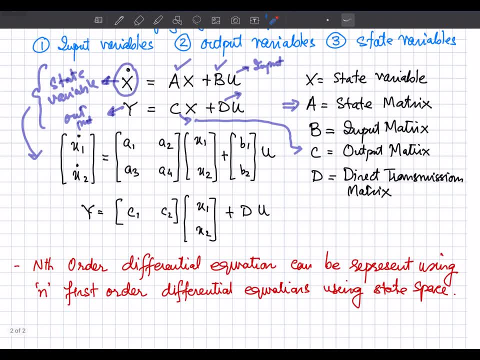 the nth order differential equation into n first order differential equation using the state space. okay, so now we will see that, how we can represent a state. sorry, a differential equation in terms of state space means n first order differential equations. now let us see how we can represent a third order. 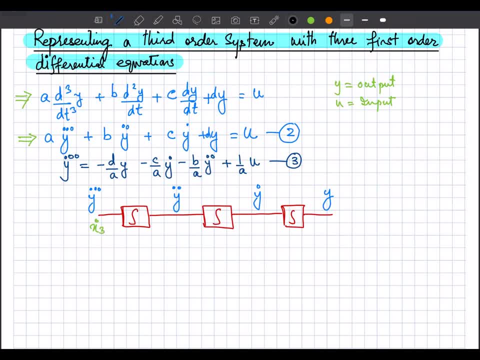 system with the first, with three first order differential equations. so let's suppose that this differential equation is there: a, the third derivative of y plus b, second derivative of y plus c, first derivative of y plus d into y, that is equal to the forcing function u. so y is the output in this case and u is the input or our forcing function. so this equation, 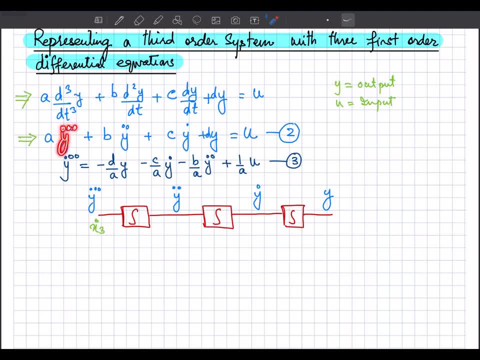 can be written like that: y three dots, where these three dots are represented the derivative y double dot, it is representing the second derivative, y dot: it is representing the first derivative. so now, if i eliminate, if i, and take out y triple dot on one side, so i can represent this equation like this: that y triple dot will be equal to minus d by a into y. 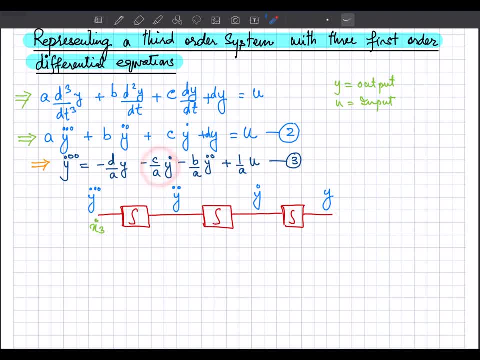 minus c by a into y, dot minus b by a, y, double dot plus 1 by a into u. so is equal to minus pi by b. so there is no Jeffrey three years on the screen all together. now, if i make do all these ridiculous because i want to possibly. 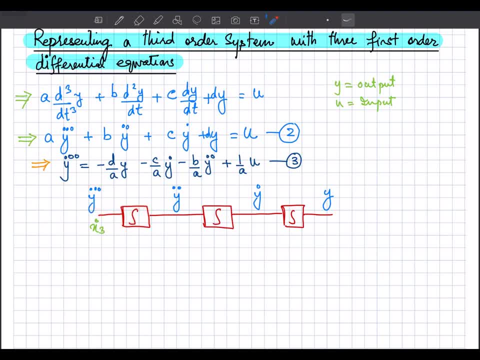 represent a wholeizer the points. what we will see was that get a y at the output. So to reach from y triple dot to y we will be requiring three integrators. So there will be three state variables for this system. The number of state variables are usually. 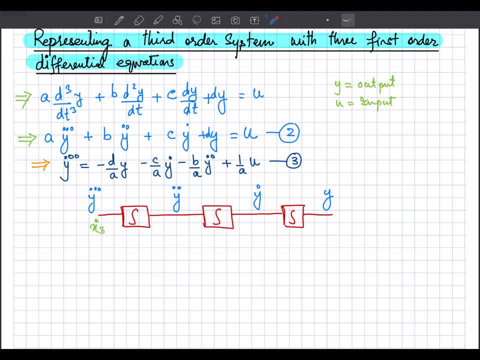 equal to the number of integrators required to implement that differential equation. Okay, so let's suppose that this output y is equal to x1, where x1 is our state variable. Then let's suppose that this is equal to y, dot is equal to x2 and y double dot is equal to x3. 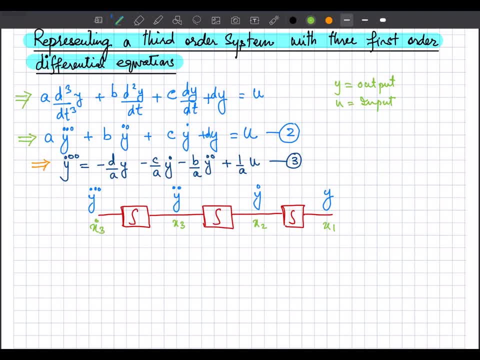 These are our three state variables. What will be the relationship between these variables? This x2, when integrated, will give you x1.. So I can say that in reverse there will be the relation of the derivative Right. so in forward, if x2 is integrated, we get x1.. 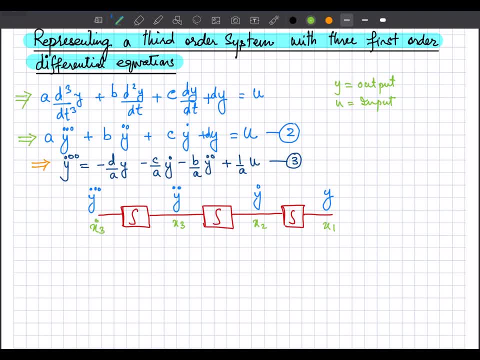 Okay. so now, if I look at this equation 3 over here, if I want to represent it with the help of the block diagram, how I can do it. So here you can see: this y triple dot is basically the summation of all the integrators. So if I look at this equation 3 over here, if I want to 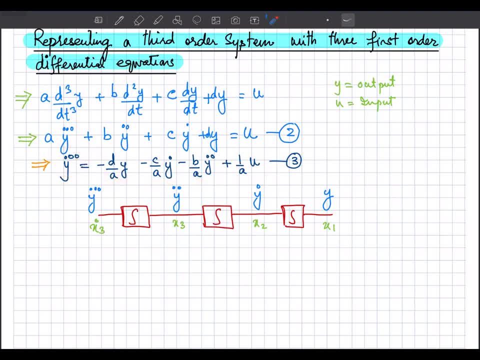 represent all of these terms, these four terms. Okay, so I am going to add, first of all, let me change the marker. Okay, so let's suppose that we have a summing block over here, Right, and the output of that summing block is y triple dot. So what that summing block will be doing, it should. 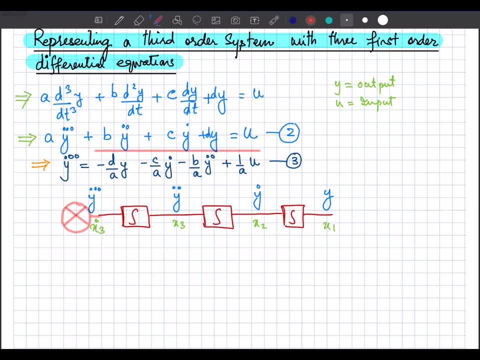 add all of these four terms Right. So it is taking y as an input, with the gain d by a. So what I will have to do, I will have to multiply this y with d by a And then y dot will be multiplied with c by a and y double dot will. 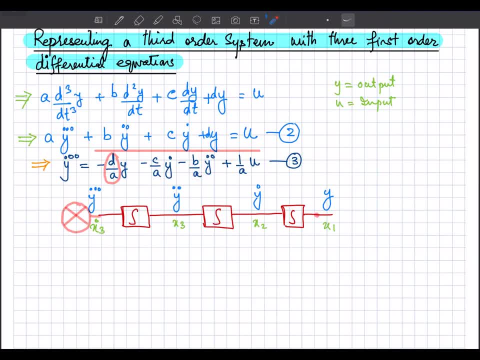 be multiplied with b by a. So let's start from y double dot. So how I can implement this one, I will be taking- let me select this: Okay, so I will take this signal, y double dot, and I will multiply it with minus b by a, and that will. 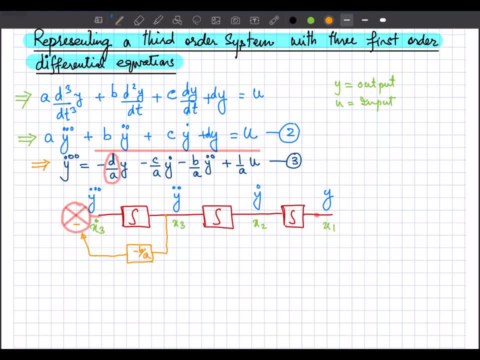 be fed to this summing node, And let's suppose that this is the negative one and this one is the positive. So whatever is coming from here, from that this will be subtracted. And what is this? this is basically minus b by a into y. 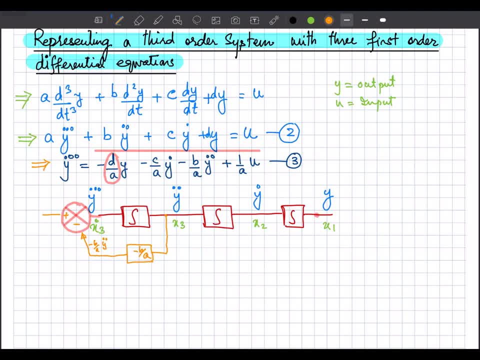 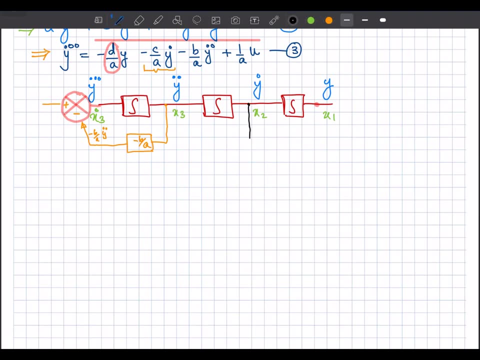 double dot. right, So I can represent it like this. Okay, then the next term is this: one minus c by a into y double dot. So how I can represent in terms of block. Okay, so y dot is available over here, So I will have to take the branch from here and the gain of this term is: 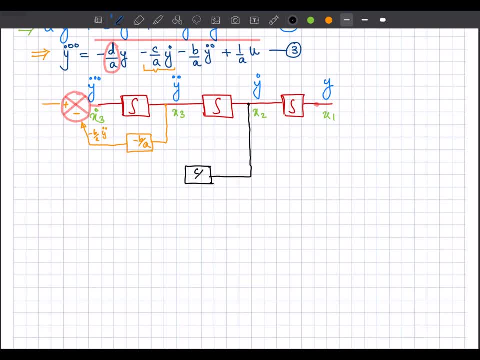 minus c by a. So I will have to write it c by a And this will be positive over here, because we are considering the negative sign over here, right? So this must be considered: plus b by a, y, double dot and negative sign. So it will be. 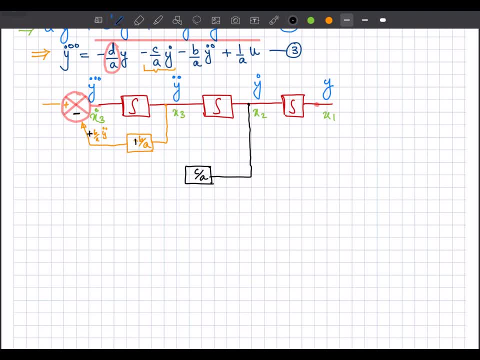 minus over here, It will become negative over here. So the gain of this y dot will be c by a and this c by a will be, when multiplied with y dot, what we are going to get. We are going to get y dot into c by a, So that should be subtracted. So again it is going into this negative. 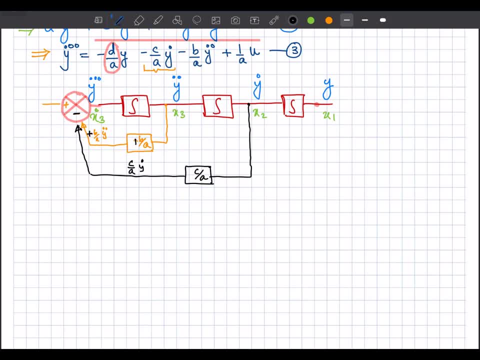 terminal of the summing block. And then we have this d by a into y, right. So y is coming from here, y is available at this point, So I am taking the signal y from here and I am going to pass it through a gain or the transfer function. that is simply equal to d by a. 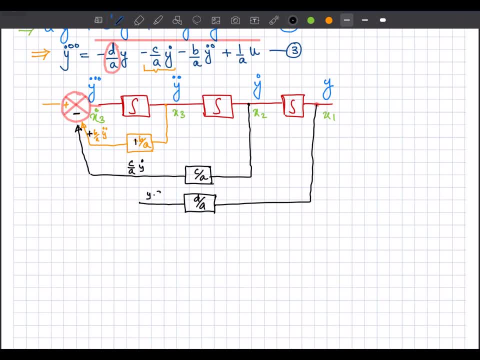 So our output will be y into d by a, And that is again fed to this negative terminal. Okay, So we are going to. we have basically implemented these terms with the help of this block diagram. What next to be added with this one, That is, this term: 1 by a into u. What is u? u is our input. 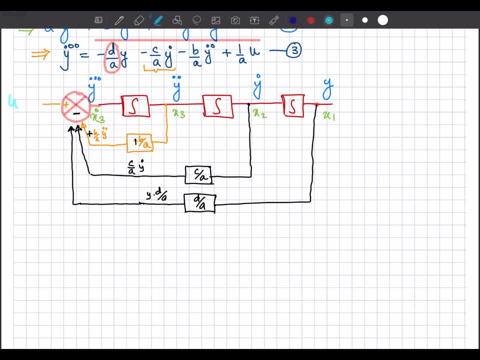 So let us suppose that u is our input And then this u will be multiplied with 1 by a, So the gain over here will be 1 by a. So the signal at this point will be u by a. So this is positive. As you can see over here, this is positive. 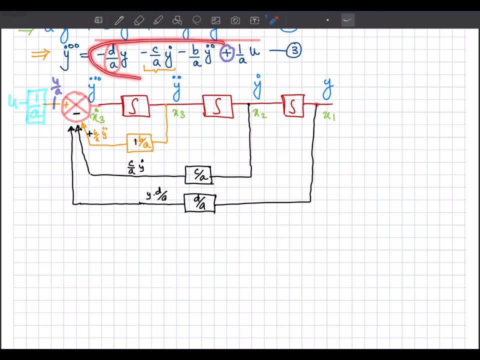 And from this all of these terms will be subtracted. So those are being subtracted over here, right? So this differential equation, this equation that is represented with equation 3, it can be represented with the help of this block diagram. 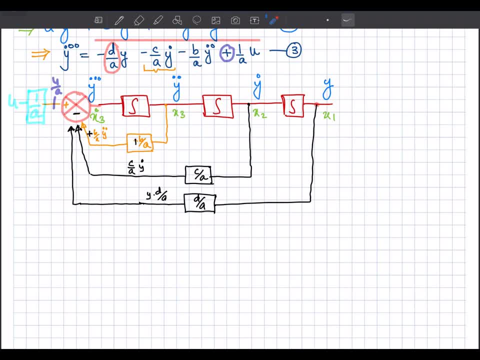 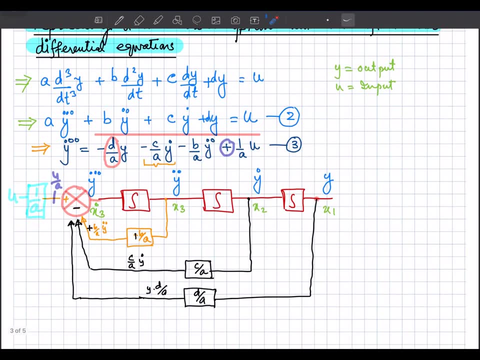 Okay, Now let us say represent it in terms of state space equation. So for that, we are going to first of all define our state variables. And what are our state variables? x1? So our output y is equal to x1, right? So from here I can say that. 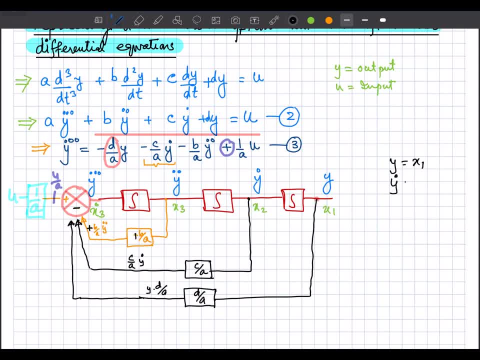 if I take the derivative of this one y dot, so this will become x1, dot right, and let's suppose that this x1 dot is equal to x2. and if I take one more derivative, y double dot, so this will be equal to x1 double dot. that will be equal to x2 dot. and let's suppose 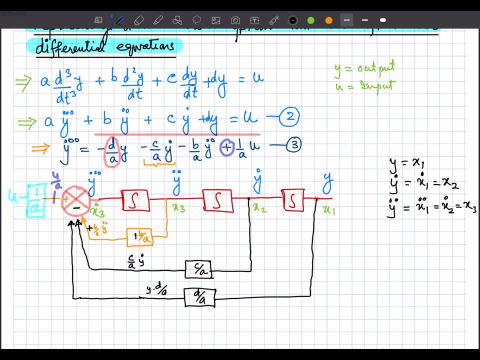 that this is equal to x3, right? so if I take one more derivative, y triple dot, so that will be equal to x3 dot. so our state variables are x1, x2 and x3, because there are three integrators, so three state variables. now we are going to write three first order differential equations. those will be: 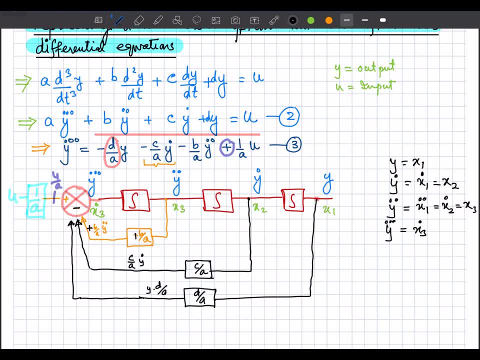 representing our this third order differential equation. so first of all, from these equations I can say that x1 is equal to x1, dot is, is, is, is is equal to x2. right, I can write it from this equation, so let me call it equation 1. and then what it is. it is the first order differential. 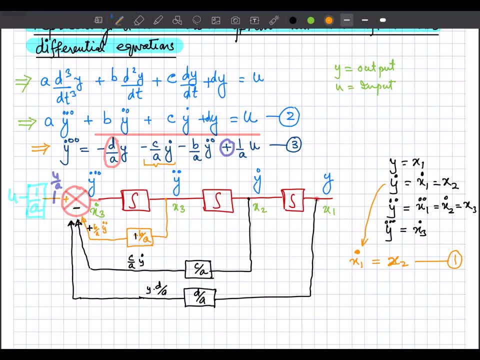 equation because we have one derivative, dx1 by dt, that is equal to x2, right? so it is a first order differential equation and from the second equation, from here I can say that x-m, x-1 dot that is equal to x3. so let me call it. 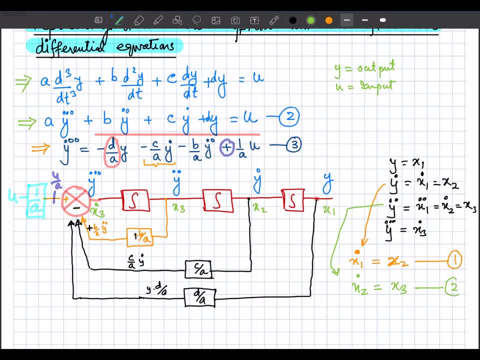 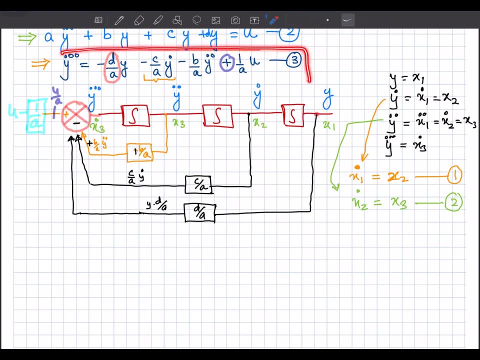 it is again first order differential equation and to write term, the third first order differential equation, I am going to use this equation, equation 3. so from this equation 3I can write that x-m, x-2 dot is equal to x3 dot, x 3 dot, because x 3 dot is equal to y triple dot, So x 3 dot will be equal to. 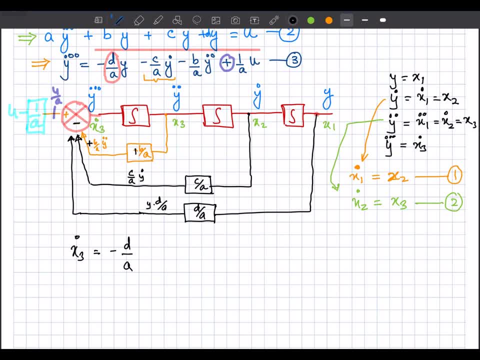 minus d by a into y. So what is y? y is equal to x 1 from this equation from here. So I can write it like that: x 1 minus d by a into x 1, then minus c by a into y dot. So what is y dot? 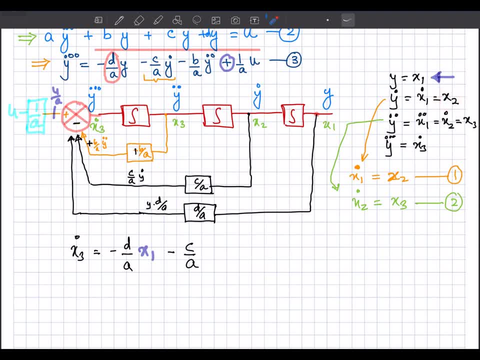 y dot is equal to x 2.. So I can write it like this: minus c by a into x 2, then the third term over here, that is minus b by a into y double dot. So now how to write this: one minus b by a. 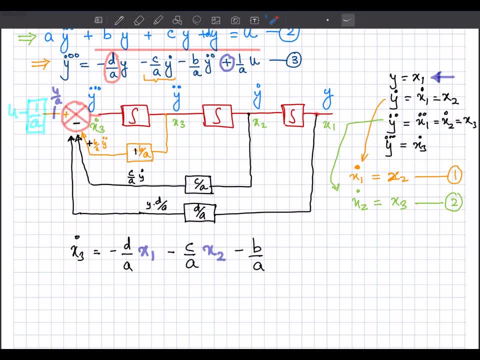 y double dot, double dot and y double dot is equal to x 3 that you can see over here. So multiplying this one with x 3, right. and then finally the input term, that is 1 by a into u. So 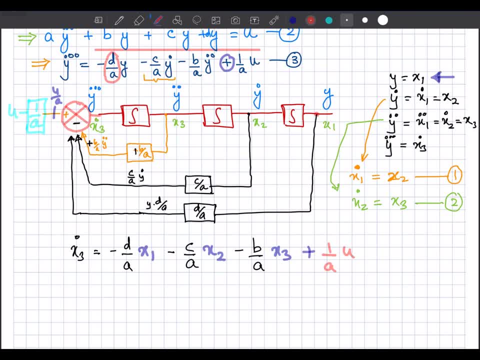 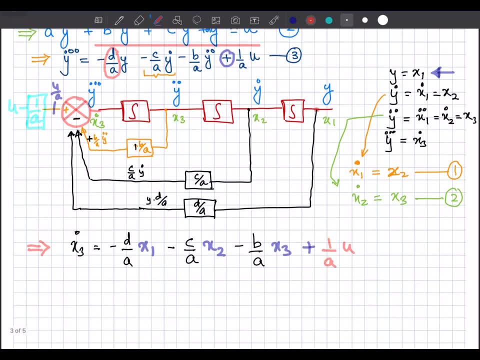 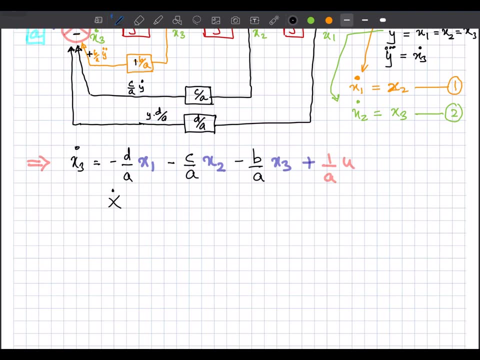 the third differential equation. first order differential equation, because you can see, only one derivative is over here: x, 3 dot. that is this one representing this system. So what is the standard form of our state space equation that is equal to x dot where x is. 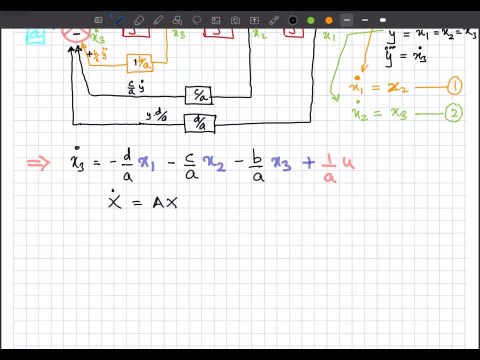 the state variable vector, that is equal to a into x plus b into u. and our output equation, y is equal to c into x plus d into u, where a is the state matrix, b is the input matrix, c is the output matrix, d is the direct transmission matrix. So now we have these three equations and we can write. 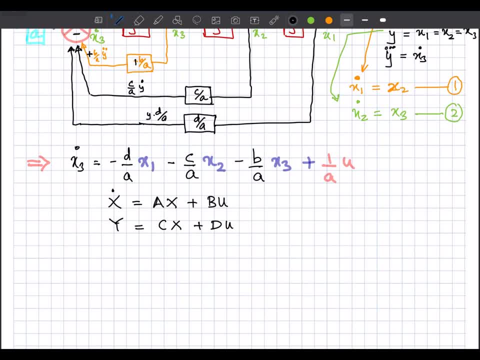 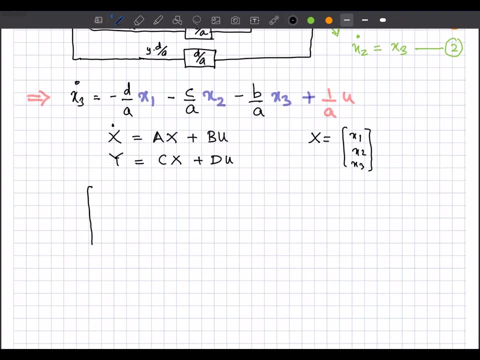 it in the standard state space form. So what we can do, what is our vector x? This vector x is basically equal to x 1,, x 2 and x 3.. These are our state variables, those we have selected over here. So now I can write it like that that this is x 1, x 2 and x 3, and 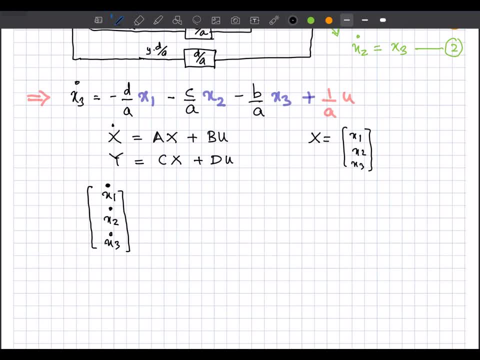 all of these are with the dots because we are taking the derivatives over here. that is equal to some matrix. This is matrix A and definitely it's order will be three cross three, because we have three state variables into x, x matrix, x 1, x 2 and x 3, then plus. 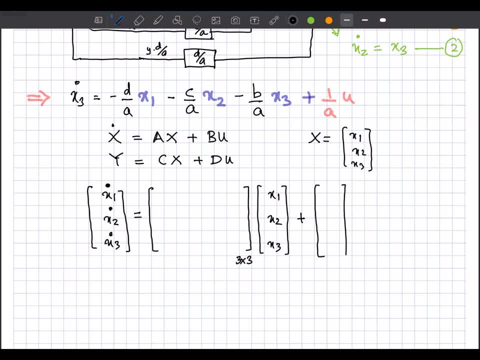 b into u. So we have one input. So there will be one column over here: x 1 into x 2, x 3 into u. So we have one input. So there will be one column over here: x 2, x 3 and there. 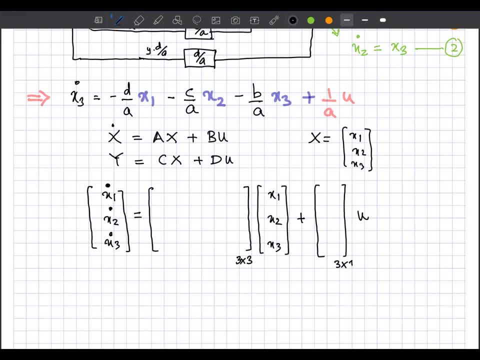 will be one column over here. So now what we can do is we have all the input, so we can. Okay, so this will be of 3 cross 1, right, and then we have output that is equal to some matrix C into state variable matrix or vector over here: x1, x2 and x3, right plus D into 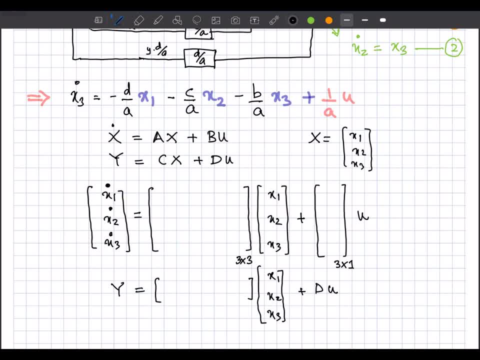 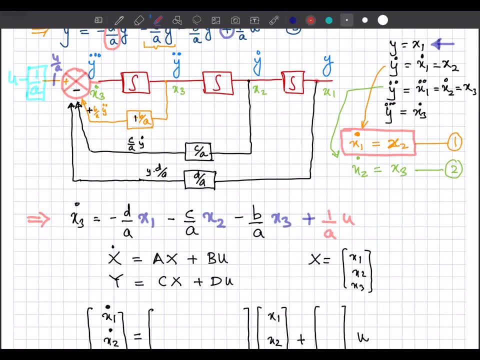 u. Okay, now let's fill the entries over here. So, first of all, taking this equation, that x1 dot is equal to x2, right? So x2 term will be 1 over here and the other terms will be. 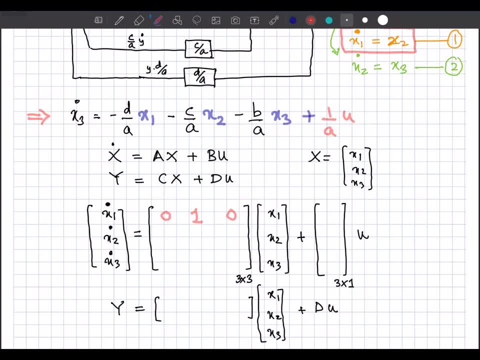 0 because x1 and x3 is not there in this equation. Now taking the second equation, that is this: one x2 dot is equal to x3.. So from this equation I can say there should be 0, 0 over here. 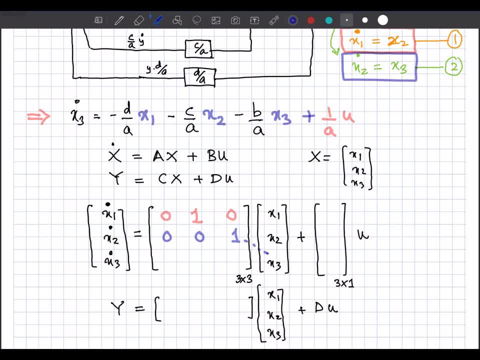 And from this equation, let me call it equation 3.. Now what I can write: with x1, I should have minus D by a, then with x2, I have minus C by a, and with x3, I have minus B by a. And with the 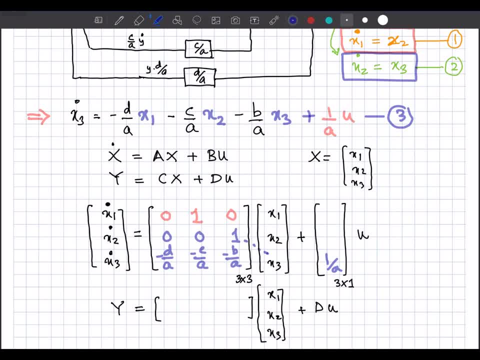 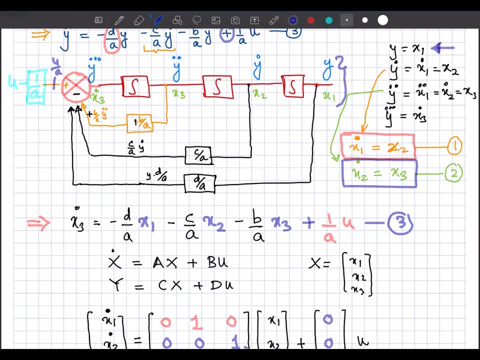 input. I have 1 by a. The other state variables x1 dot and x2 dot. those are not linked with the input, So there will be 0s over here And the output. the output is equal to x1. that you can see from here. 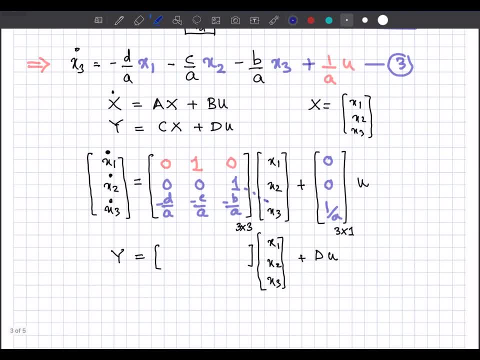 So x1 is to be obtained at the output, So there will be 1 over here. x2 is not there, So it will be 0 and 0.. So when you will multiply this matrix 1 cross 3 with this 3 cross 1,. 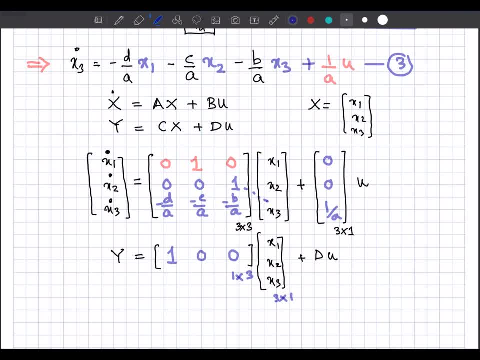 so the resultant will be 1 cross 1.. So the output will be x1. And in this particular case this output is not linked with the input, So D is equal to 0.. So this is the state space form. 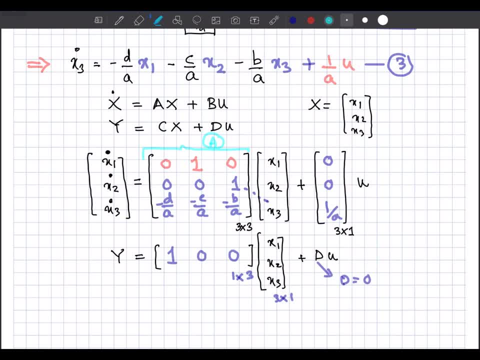 of the differential equation. This is our matrix A, the state matrix, This is the x And this is our input matrix B. This one, this one is the input matrix, And then we have this output matrix. So output matrix for this case is 1 double 0 and the direct transmission matrix that is equal to. 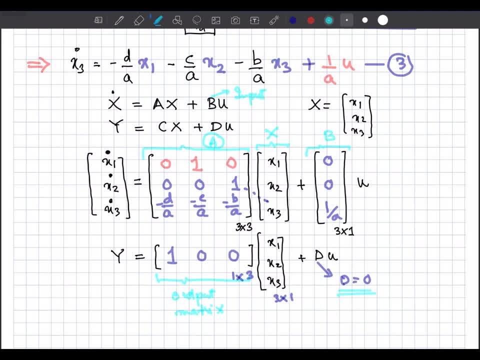 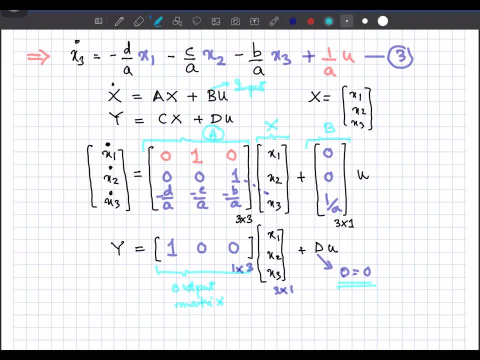 0 in this case means your input is not directly transferred to your output. So you have seen, we have represented a third order differential equation with three: first order differential equation- This is the first equation. second equation and the third equation given by this row of this multiplication. Now let us quickly go through the state space. 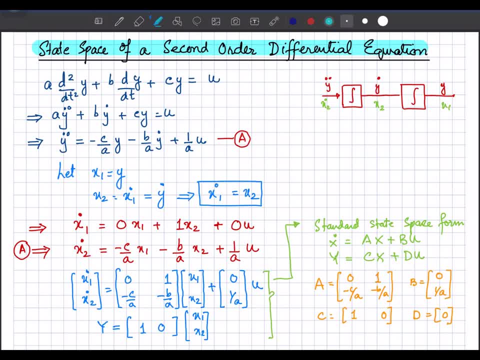 representation of a second order differential equation. So let us go through the state space. representation of a second order differential equation. So here you can see the differential equation: A into the second derivative of the y plus B into first derivative of the y plus C into y. 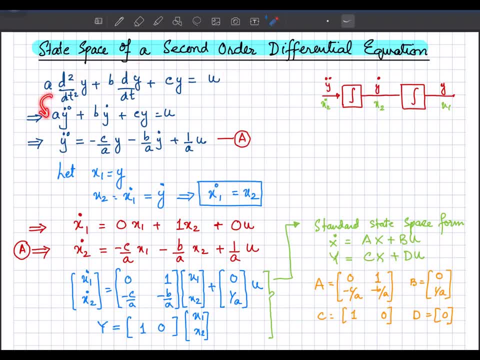 that is equal to our forcing function u. And I can write this equation like this: A y double dot, B y dot plus C y, that will be equal to u. And this from this equation. if I expect y double dot, I can write it like this: Okay, So here you can see if y double dot is given to this: 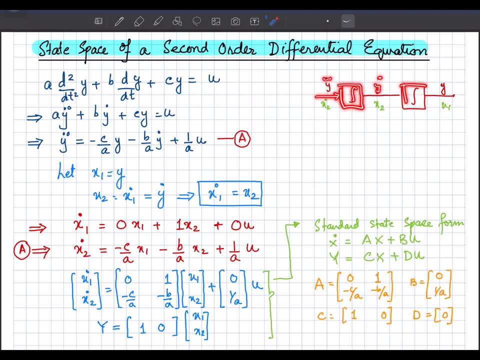 integrator we are going to get y dot, and if that is passed through an integrator we will be getting y. So let us suppose that this y is equal to x1, this y dot is equal to x2.. So two state variables. 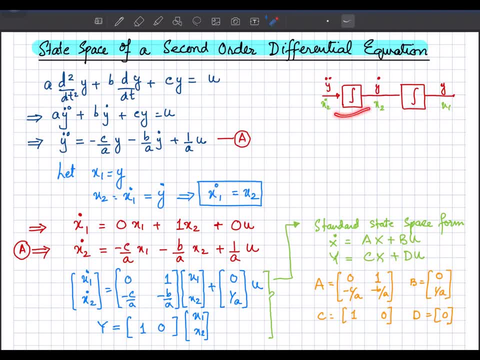 are required because there are two integrators. And over here, if I want to relate with this one, this will be x2 dot, because x2 dot, when integrated, you will get equal to x2.. Okay, So let us define x1 dot, So this will be equal to y dot. Okay, From here and from this equation, I can say that 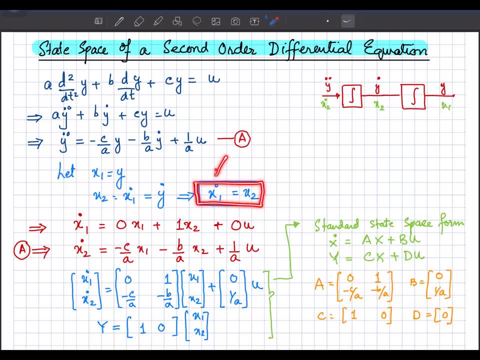 x1 dot is equal to x2, the differential equation of our first state variable. Okay, So from this equation I can write like that: x1 dot is equal to 0, x1.. It does not depend upon x1,, but it simply. 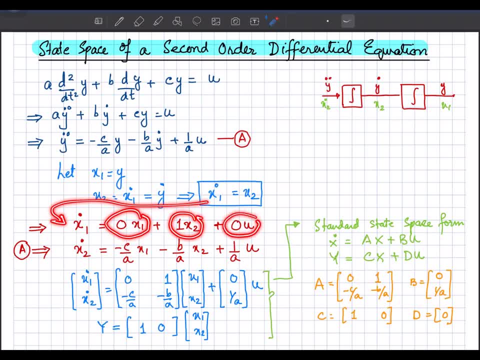 depends upon x2, 1 x2 and it is not linked with the input. So 0 u. And for the second equation I am going to use this one: y double dot that is equal to x2 dot. So x2 dot is equal to minus c by a into y And we want to write it in terms of state variables. So 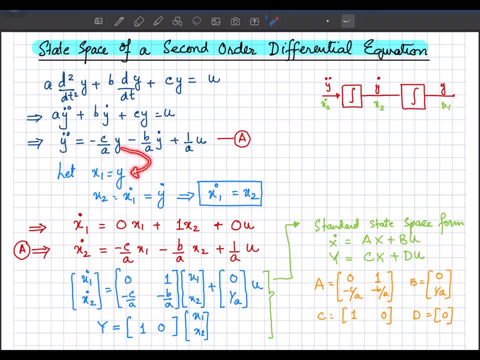 this y will be written in terms of x1 like that: So minus c by a into x1.. Then the second term, minus b by a into y dot. So minus b by a into y dot, and y dot is equal to, in terms of state variable, x2.. So I am going to. 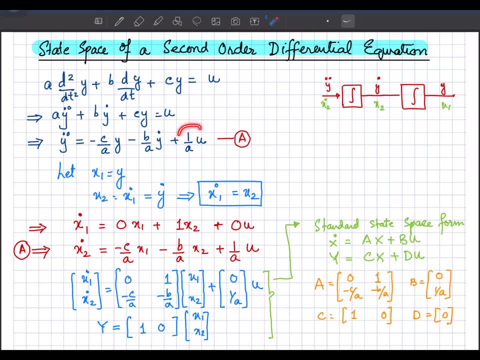 write it like that: minus b by a into x2.. And then the input term 1 by a into u. Okay, So we can write it in terms of matrix equation: x1 dot, then x2 dot. This is going to have represent. this is: 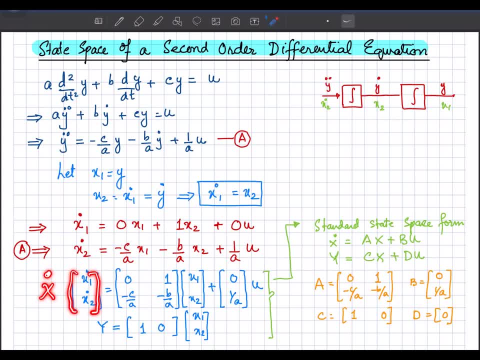 x, dot right, The derivative of the state variable. Okay, So then these terms, okay, over here. from here I can say 0, 1 minus c by a, minus b by a, against state variable x1 and x2, and then plus 0 and 1 by a into the input u, And what is the? 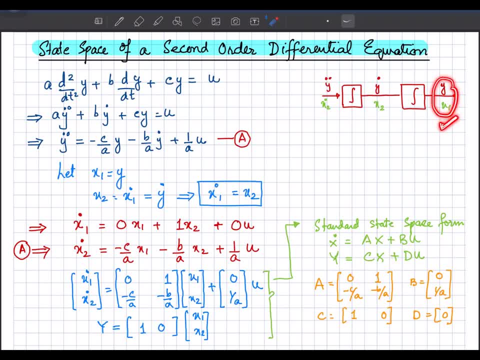 output. Output is equal to x1, right? So y is equal to x1.. So here you can see, x1 will be multiplied with 1 and x2 will be multiplied with 0. So this is our output. 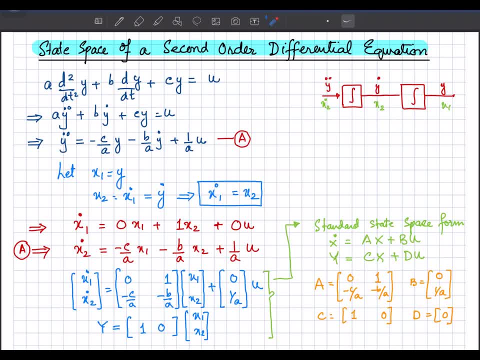 equation and the d in this case is 0, right. So if we compare it with the standard state space form, x, dot, that is equal to ax plus bu and y is equal to cx plus du. So I can say that a is: 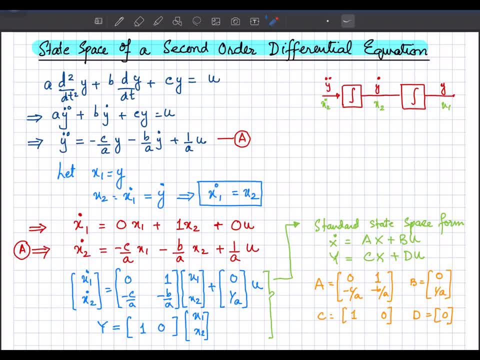 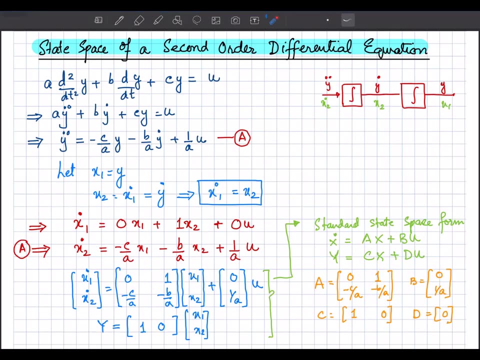 equal to this matrix: 0, 1 minus c, by a minus b, by. This is our state matrix, This is our input matrix, obtained from here, and this is our output matrix, and d is equal to 0 in this case. So we have represented first- sorry, second order- differential equation with: 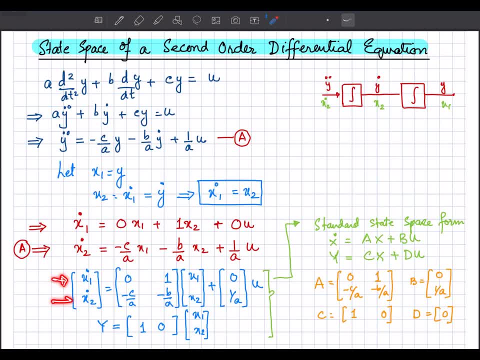 two first order differential equations. Okay, So that is the concept of the state space. Okay, Now let us complete this block diagram quickly. If we look at this equation a, so y dot is equal to the sum of all of these terms, right? So, first of all, 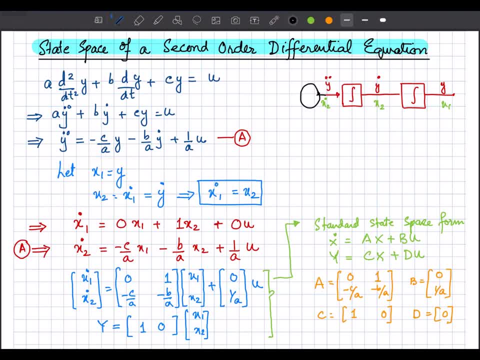 we need to have the input u. So let us suppose the input is this: u. So this is to be passed through the gain, and that gain is equal to 1 by a. So 1 by a over here that will be. 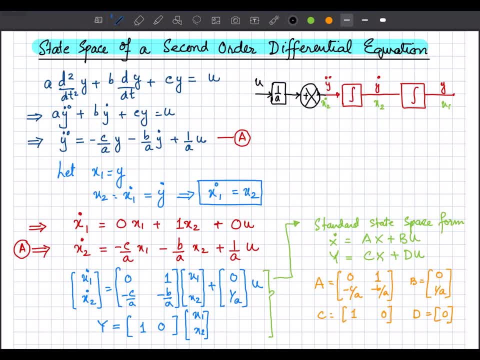 fed to this summing block and this is positive, As you can see the positive sign over here and all other terms are negative, So negative sign will be used over here. Okay, So y dot, y dot is multiplied with b by a and then fed to the negative terminal of your summing. 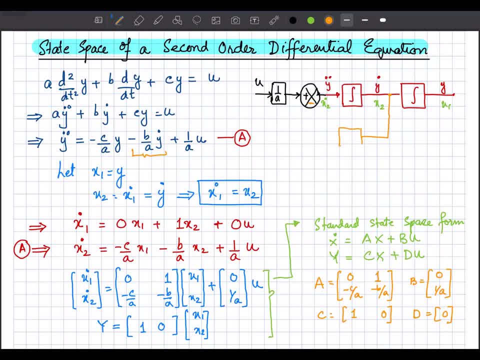 So y dot is taken from here and what we have? we have the gain of b by a over here, going into this summing block at the negative point. Okay, So then the next term is this one y into c by a, So we can take this one y from here and the gain of this. 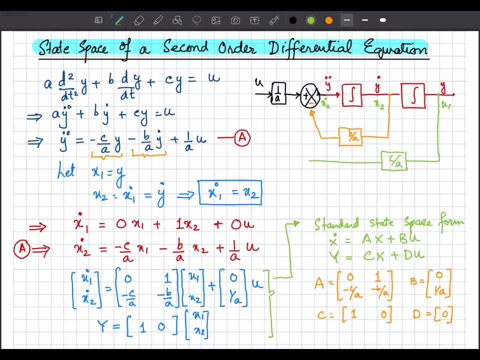 will be equal to c by a, and this will be fed to the summing block. You can use the positive sign over here and you can represent the negatives over here, indicating that these signals will be negative, and then in that case you will have to add the negative signs over here. Otherwise. 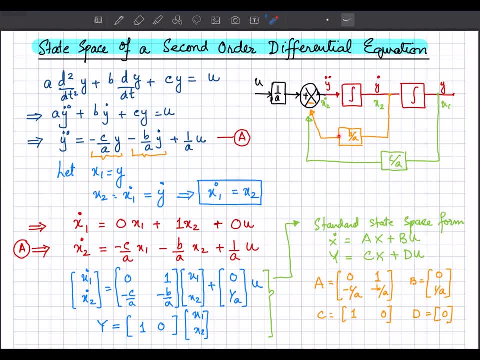 if you are using negative sign over here, there is no need to take. this will be the positive one. Okay, So this is the block diagram representing our this second order differential. So this is the block diagram representing our this second order differential. 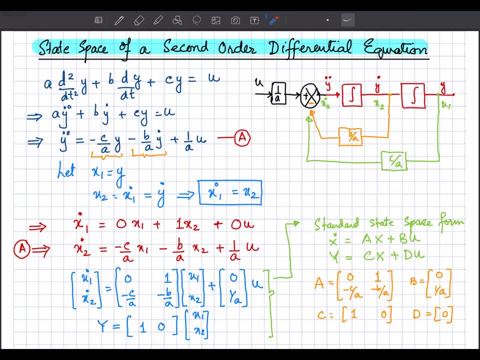 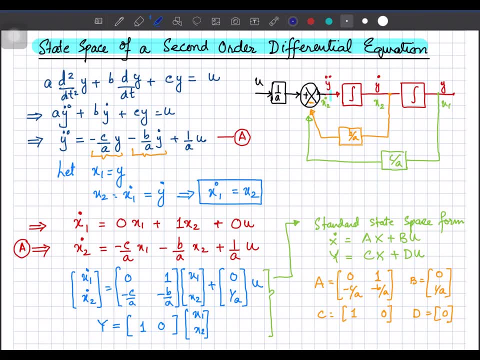 equation. So here you can see that y double dot is given by this equation, minus c by a into y, and you are getting this term from here in this loop. This is the loop: y into c by a right and then y dot into b by a. this is going towards this negative terminal and the input is coming from: